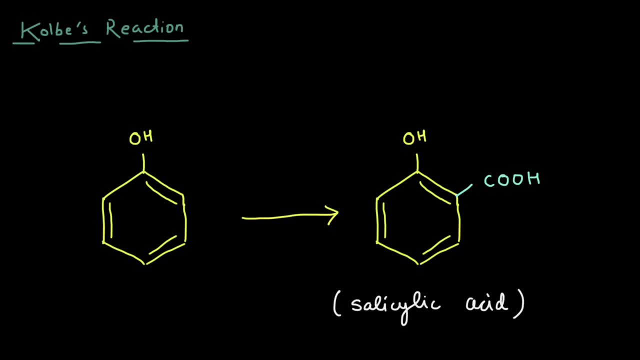 So the most important thing that I want you to know about goal-based reaction is that we're going to be starting with a phenol and our end product is going to be salicylic acid, which is basically a COOH getting added to the ortho position, and this reaction is important for. 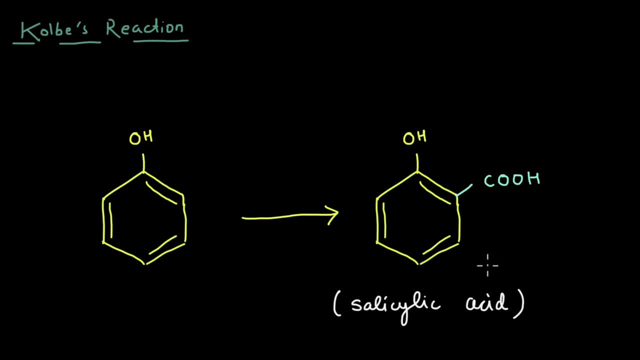 many reasons, One of which is that salicylic acid is used to make aspirin, which is usually prescribed by the doctors when you have minor pains or fevers or things like that. So that's why this reaction is important. So I've told you what the end product is, but I haven't told you. 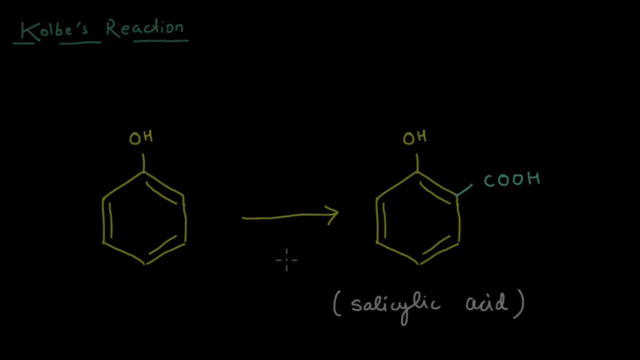 what the reagents are or how we get from here to here. So let's see that. So I've broken down the reaction into two steps. The first step is reaction with NaOH and the second step is reaction with CO2 and the addition of an H+, And you can probably see what's happening in these reactions, Like in: 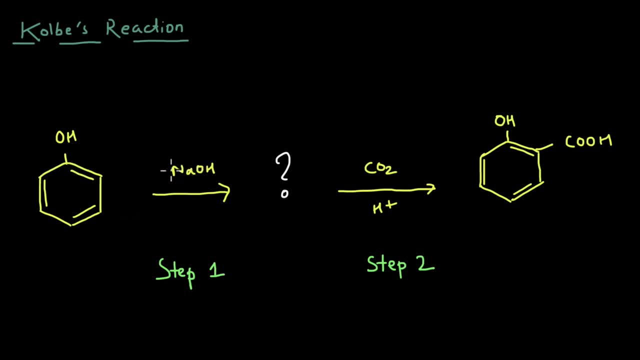 the first step, NaOH is a base and phenol is an acid, So this is an acid-base reaction. and in the second step, there's a CO2 here. So maybe this is what is going to be a part of the COOH here. So let's see how this happens. But before we go to the reaction, 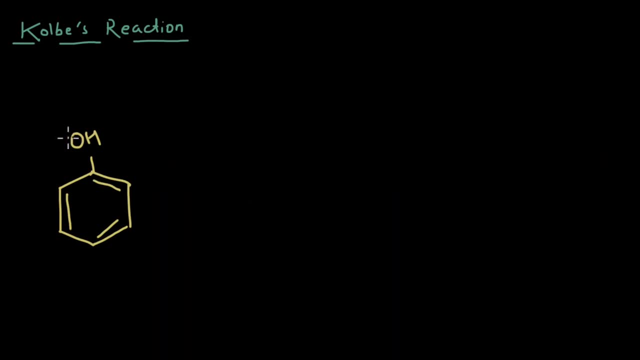 there's something to know about phenol. So, as you know, this oxygen here has lone pairs that it is going to share with the ring, because of which the electron density in the ring increases, And because of resonance, the electron density is higher at the ortho and the para positions. So let's see. 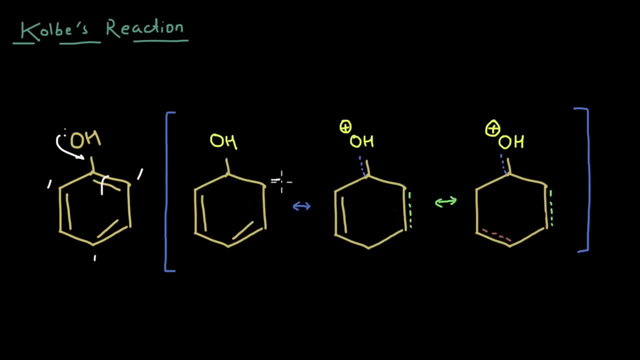 how the resonance happens. Now, if we break this double bond, we know that there'll be a negative charge here and a positive charge here, But there's also an oxygen atom here. So what's going to happen here? on oxygen, a double bond is going to form here and there's going to be a positive charge on this. 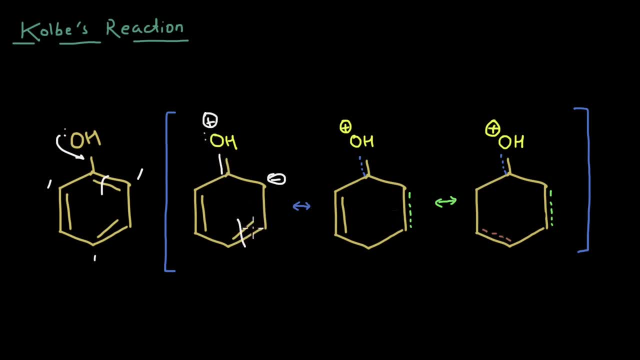 oxygen atom. Next, what we can do is we can break this double bond, because of which there will be a positive charge here and a negative charge here, And you can see that the negative charge here from before and this positive charge forms a double bond here. And lastly, if we break this double bond, 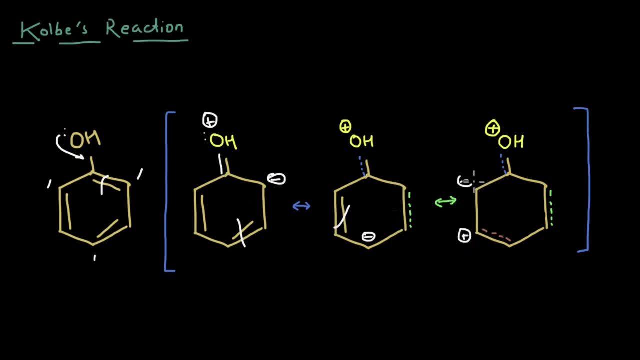 we can see that there will be a positive charge here and a negative charge here. So this positive charge along with this negative charge will form a double bond here. So these are the resonance here. Now, if you follow the negative charge here across all the three of these structures, you'll. 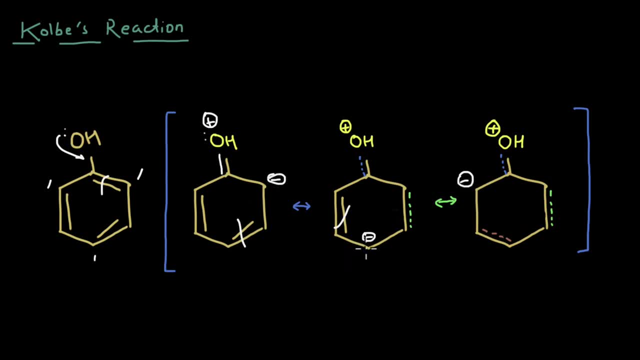 notice how the electron density is higher at these ortho positions and this para position, Which is why we say that the OH group is an ortho para directing group. So that's one thing about phenol. So we saw how the phenol is ortho para directing. Now let's think about what happens if this. 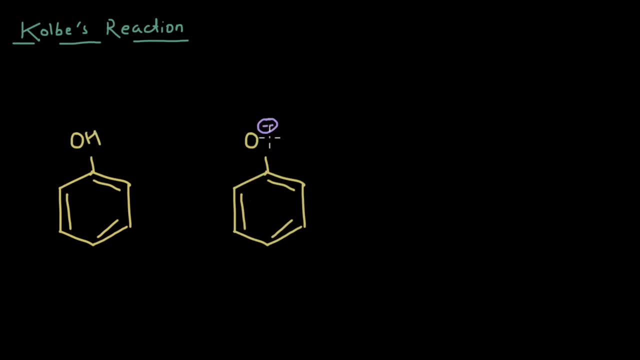 hydrogen is taken off. So if we take off the hydrogen, what we get is this phenoxide anion. Now, the idea here is that once we have taken off the hydrogen and there is a formal negative charge on this oxygen atom, it makes it very easy for the resonance to happen. Because here, in the case of 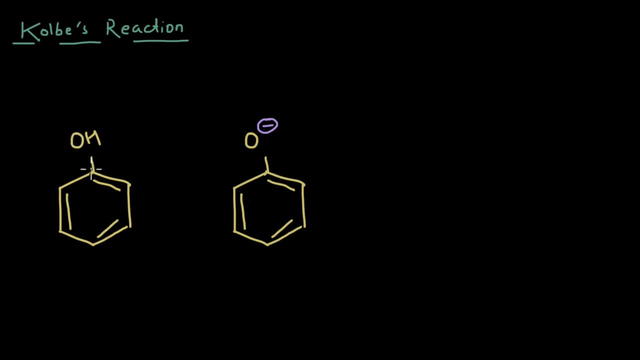 phenol, it was the lone pairs which were contributing to the resonance, So you always had a positive charge on this oxygen. But now, with the hydrogen gone, this negative charge will make it way more easier for the resonance to happen Effectively. what is happening is the phenoxide anion will be 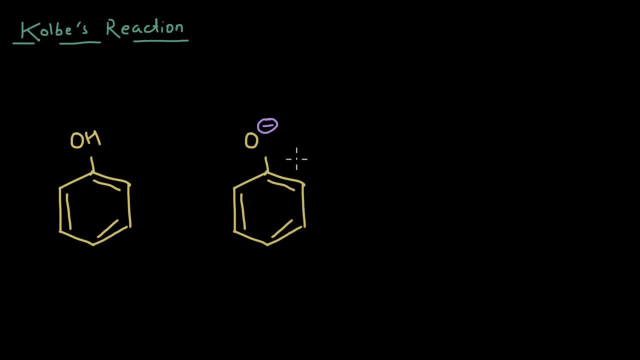 more reactive, or we could say that it is more ortho para directing, Because this negative charge is easily transferred to these ortho and para positions. So now, with this information that the phenoxide anion is more ortho para directing or more reactive, you can probably 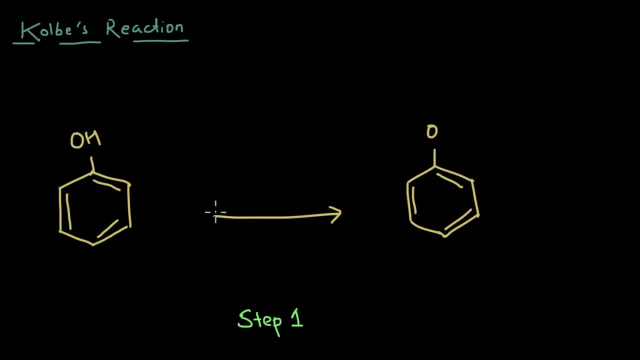 guess what the first step of the reaction is going to be. So I told you before that the first step is reaction with NaOH. Let me just write it down here and you can already guess what's going to happen. So, because we want a phenoxide ion, what this base is going to do is going to take off the hydrogen. 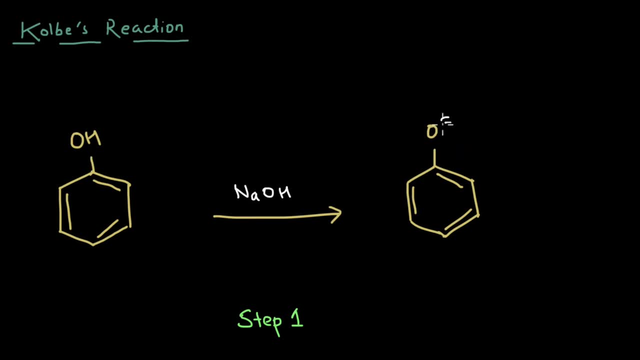 from here. So what we're going to have is we'll have a negative charge here and there will be one Na plus here, And this is actually going to be a negative charge because we have an Na plus And the is the first step of the reaction. So now, at the end of the first step, we have got this phenoxide. 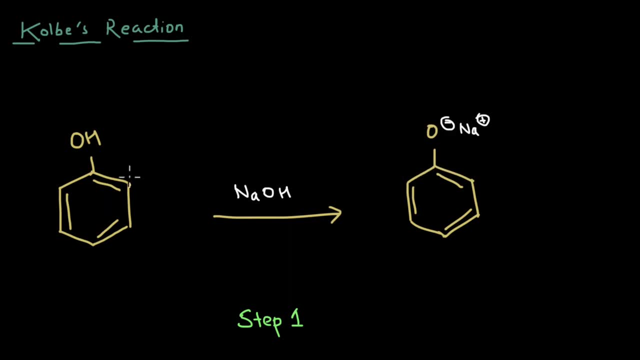 ion, which has a negative charge and it is more reactive than the phenol that we started with. And because we have this negative charge that is distributed to the ortho and para positions, this is now ready to attack in the next step. Let's see how that happens. So the second step. 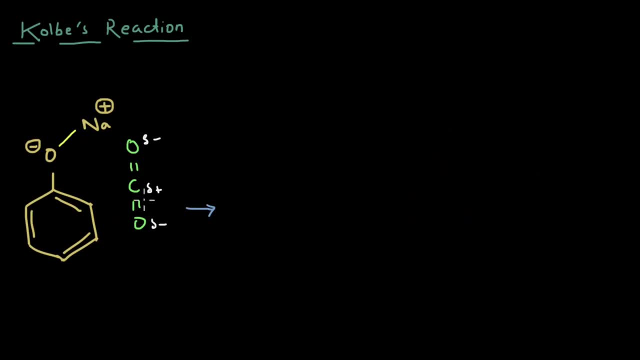 started with reaction with CO2.. So I've just written down CO2 here. it's written in a slightly different manner, But essentially what we're doing is we're initiating the reaction with CO2 here, And this is the phenoxide ion from the earlier step, which is more reactive, So think. 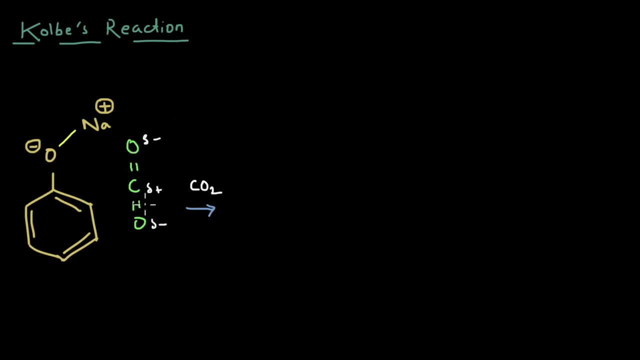 of what's happening here Now. CO2 is a weak electrophile, but we do have this oxygen pulling electrons away from the carbon and the carbon having a slightly positive charge. that's developed here, And also there is this interaction between this sodium and this oxygen, So maybe it's just. 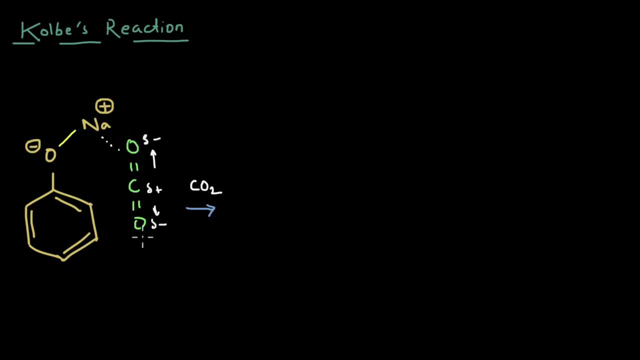 helping it align a little bit and getting it ready For the reaction. And then what happens is, because it's a phenoxide ion, let's say we break this bond and we get a negative charge here and a double bond has formed here. And because the bond 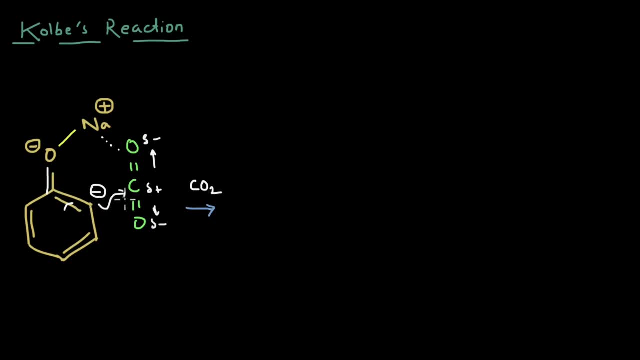 is broken, so it will immediately go and get attached to this carbon here And now. what happens is this CO2 is here and there's also a hydrogen here, And something drastic happened in this step, If you notice, the aromaticity of the ring is broken. So to quickly get back to the stability, 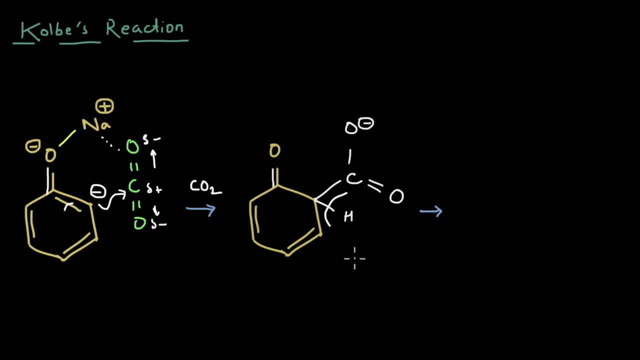 of the aromaticity. what happens is we get a negative charge here and we get a double bond here. So what happens is this H is thrown out and this bond is completed. So then what happens? We see that the H has got added here, the CO2 is here and the double bond is formed. 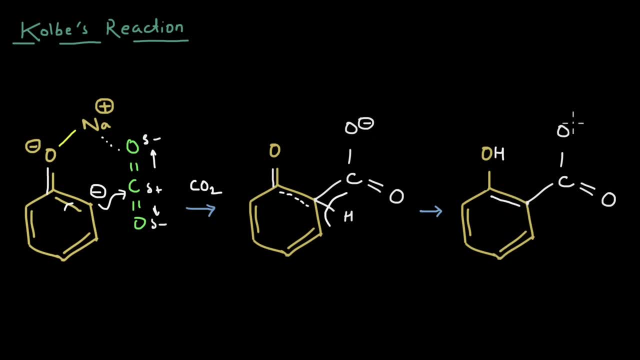 restoring the aromaticity of the ring, And of course there will be a negative charge here. So now it looks like we are almost there. There is some small thing missing. So let's do one thing: let's provide it some H+. So if we go ahead and give it some H+, it will just go and attach itself. 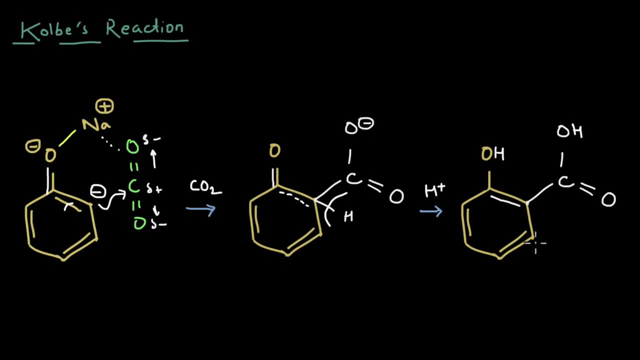 here, and we have our COOH here, which is added to the ortho position. So that completes our reaction. We started with a phenoxide ion, which was more reactive. We got a weak electrophile. for the next step, The CO2 was here, and then we got COOH. finally, when we added a little bit of H+, 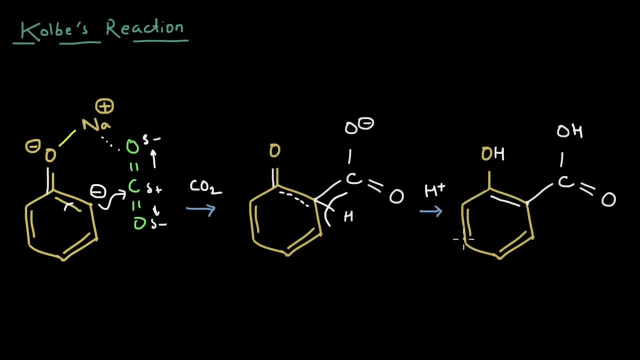 But the question is: you may remember from before that the OH group was ortho-para directing, So the electron density had to be higher at both the ortho and the para positions, which means we should have got a para product as well. So where did it go? Well, it is there. We will get some. 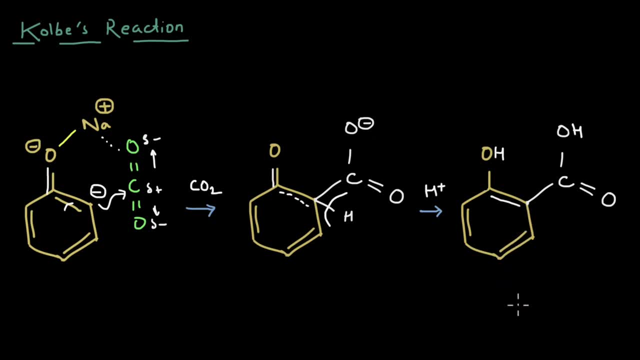 para product as well. But what we'll find is the ortho product is the major product. Let me just write it down here. So this is the major product and the para product is a minor product. Let's try to understand why this happened So usually, when you have a major product which is ortho or